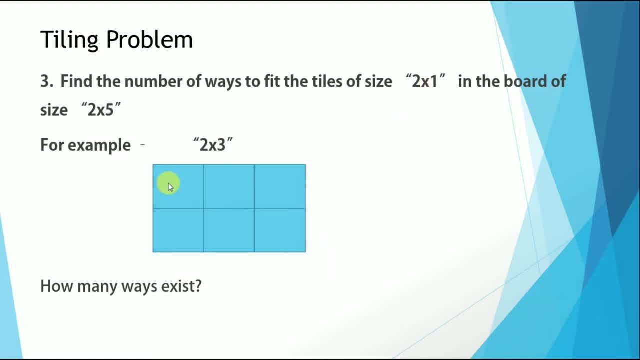 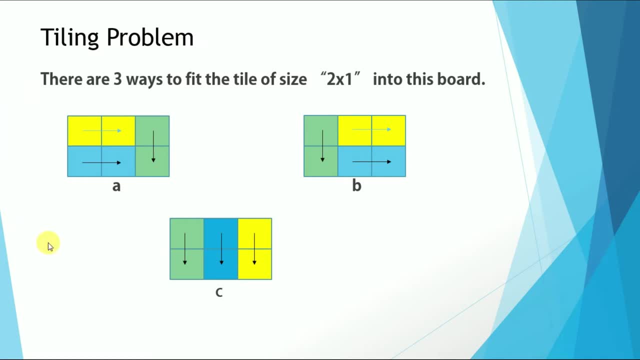 place the 2 by 1 tiles either horizontally or vertically. So how many ways exist? You can see that there are 3 ways to fit in the tiles of 2 by 1 unit in the 2 by 3 board. In the first figure, 2 tiles are 2 by 3 units. In the second figure, 2 tiles are 2 by 3 units. 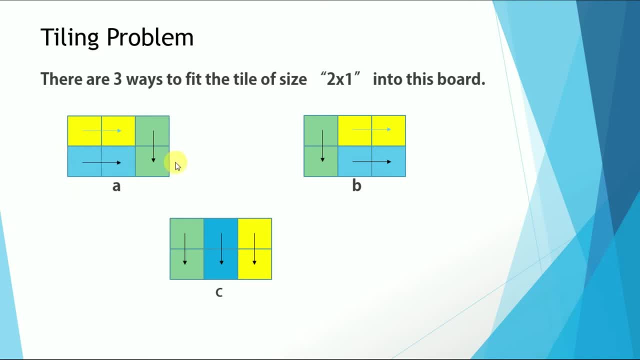 The tiles are placed horizontally first, and then the third tile is placed vertically. In the second figure first tile is placed vertically and the two others horizontally. In the third figure all three tiles are placed vertically In a similar manner. we are going. 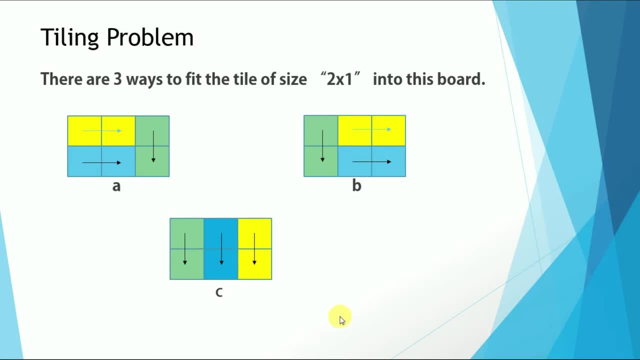 to find out the number of ways to fit 2 by 1 tiles in the 2 by 5 board in our framework. But before we switch to our framework, a humble request to you to subscribe to my channel, if you haven't done it yet, and hit the bell icon so that. 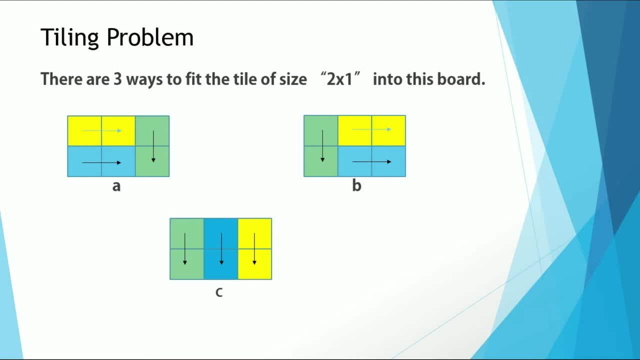 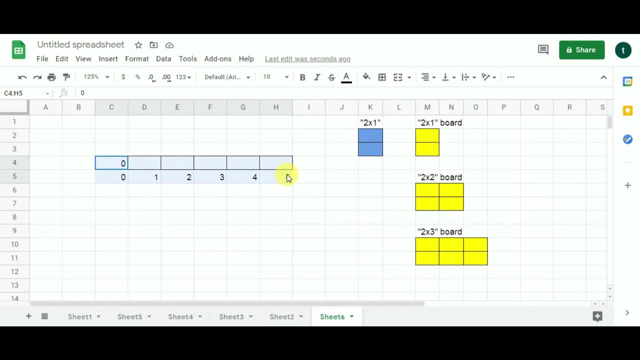 you don't miss the next video. Now let's switch to the framework and solve this classic tiling problem. This array over here is going to store the results of individual subproblems. We will begin with the smallest subproblem, which is represented by this cell indexed by 1.. This 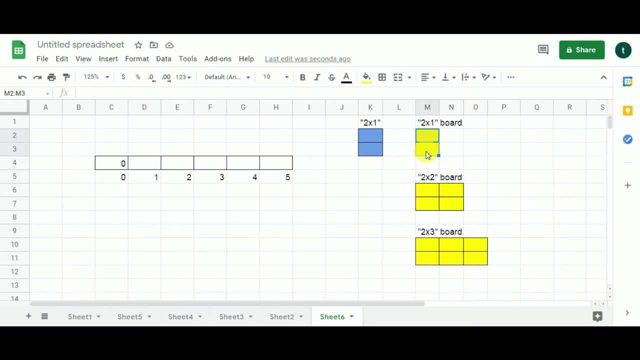 subproblem represents a board of 2 by 1.. You can see that the tile is 2 by 1 and the board is also 2 by 1.. Logically, there is only one way to solve this problem. The tile is 2 by. 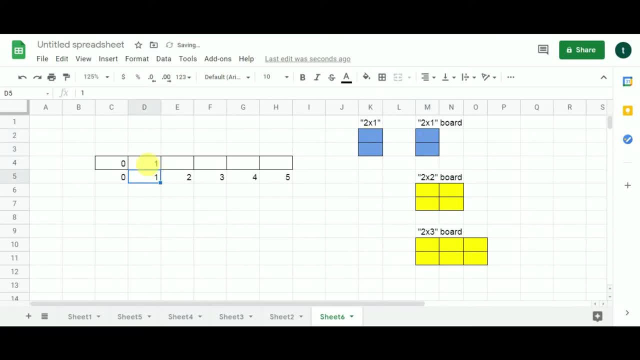 way to fit this tile in this board. So I populate 1 in this cell, 1 for the number of ways. There is only one way to fit a 2x1 tile into a 2x1 board. Now we move to the next problem, which represents the board 2x2.. Here we can fit both tiles. 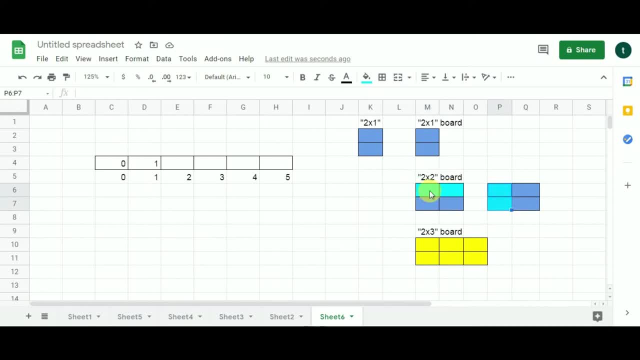 either horizontally or vertically, So there are two ways by which we can fit 2x1 tiles in the board of 2x2.. Let's check this third sub-problem. Now we have a board of 2x3.. There. 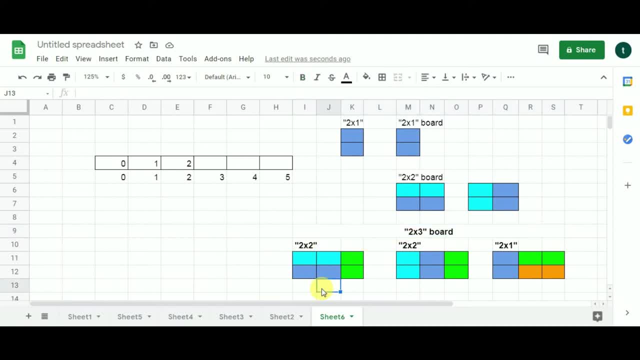 are basically three ways in which 2x1 tiles can be placed in the board of 2x3, as we saw in the previous slide. Let's check this first figure From this arrangement. if you take out this last one, which is in green, then observe the remaining arrangement, This arrangement. 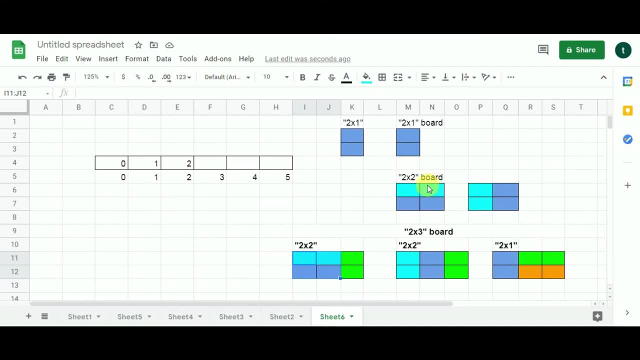 we saw for the 2x2 board. Observe that the tile we ignored for a while was placed vertically From this second arrangement. if you take out the last tile which is in green for a while, then observe again that this is the second pattern from the 2x2 board arrangements. Note again that this tile we 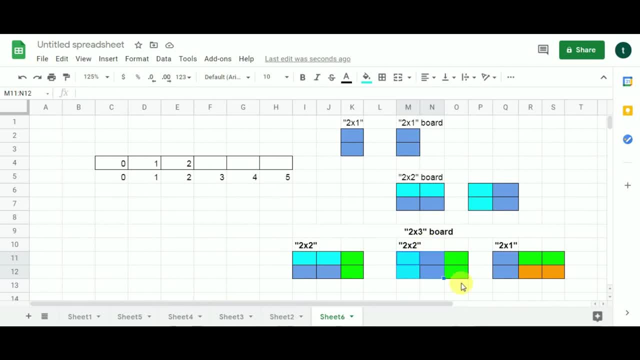 ignored for a while, is also placed vertically. This means that the number of ways for 2x3's board is going to be the same as the number of ways for 2x2's board. But wait, we have one more pattern remaining. Now look at this last arrangement. The last tile is placed. 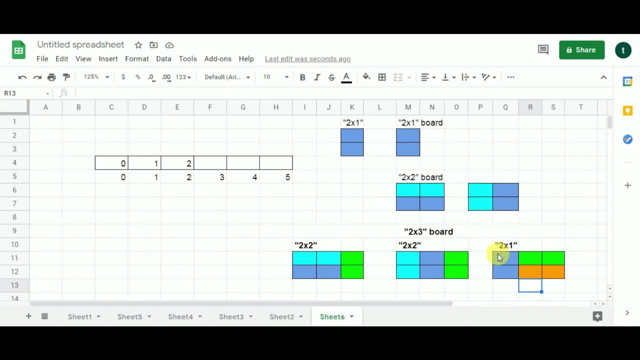 horizontally. We ignore it and see this pattern again. This is the pattern we saw for 2x1 board. We can easily say that number of ways for 2x3's board is equal to the number of 2x1's boards. 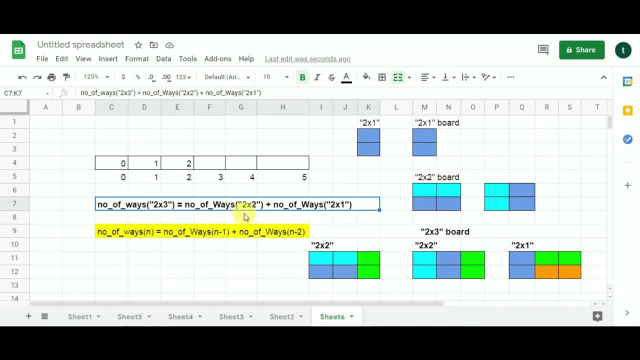 is equal to number of ways for 2 by 2 board plus number of ways for 2 by 1 board. or, in simple terms, it can be written as: number of ways for n equals to number of ways for n minus 1, plus number of. 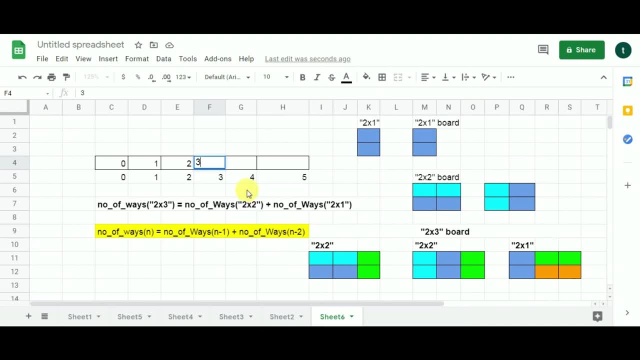 ways for n minus 2. if you see, then this is the fibonacci series algorithm, so this dp problem is solved using the fibonacci series. so we already have the number of ways for 2 by 2 tiles, and the number of ways for 2 by 1 tile is stored in our array. and this is what dynamic programming. 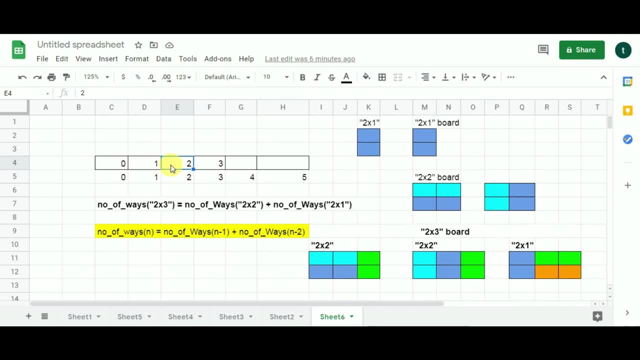 is now based on this algorithm or this formula. let's quickly fill the subsequent cells now. the next sub problem is indexed by 4, which represents a board of 2 by 4 unit. to find out the number of ways for a 2 by 4 board, we are going to use this formula: 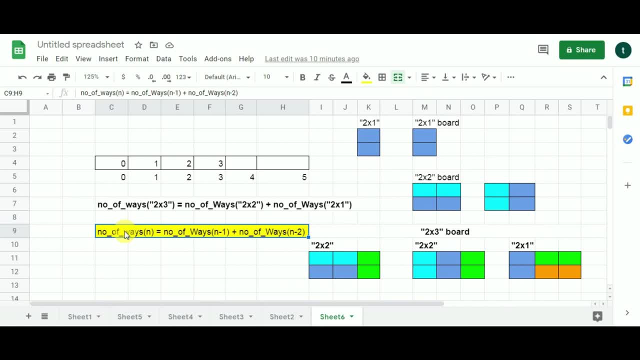 so the number of ways for a 2 by 4 board is going to be equal to the number of ways for a 2 by 3 board, which is 3 added to the number of ways for a 2 by 2 board, which is 2. so 3 added to 2 is going. 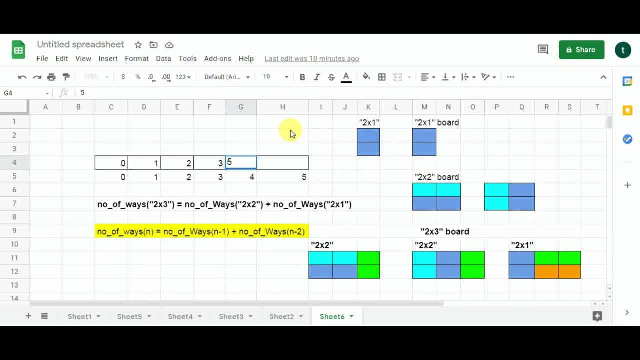 to give me 5 and that 5 i am going to populate here. so 5 is the number of ways by which we can place 2 by 1 tiles into a 2 by 4 board. the next sub problem, indexed by 5, represents a board of 2 by 5. 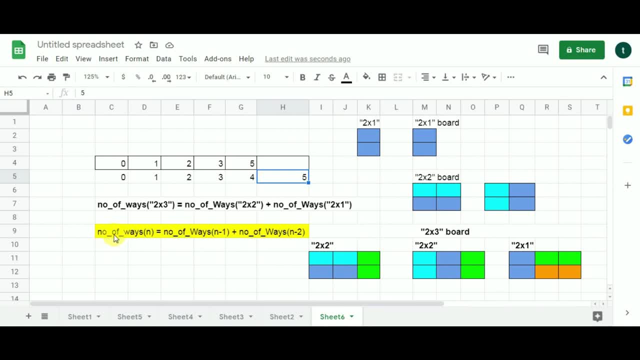 we are going to use this formula in order to find out the number of ways for a 2 by 5 board, and that is going to be equal to the number of ways for a 2 by 4 board, which is 5, added to the number of ways for a 2 by 4 board, which is 5. 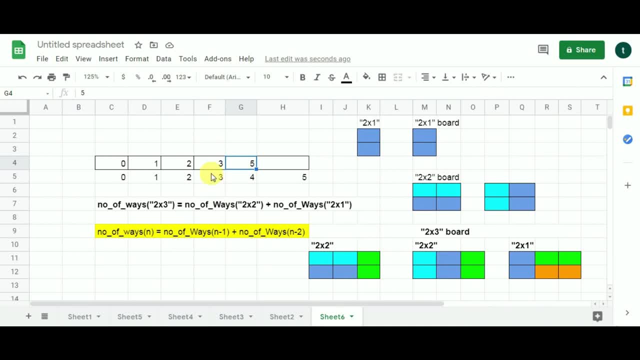 added to the number of ways for a 2 by 3 board, which is 3, 5 plus 3, is going to give me 8, and 8 is the number of ways by which we can fit 2 by 1 tiles in a 2 by 5 board. so this 8 is the answer. now the algorithm is right in front of you and 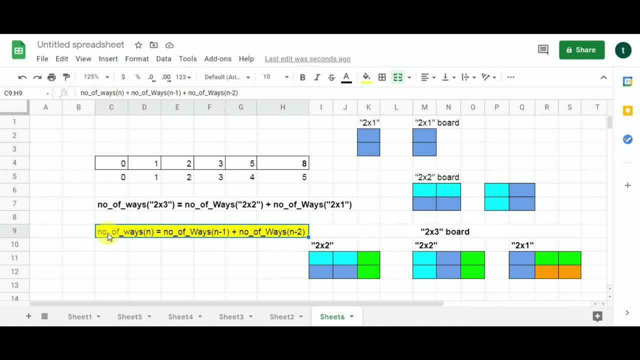 you can create a program around it in order to solve the tiling problem. if it appears in your program. if it appears in your program, next tech interview. So this concludes this video. I hope you enjoyed watching this video. I hope you learned from this video. Do give it a thumbs up. Let me know. 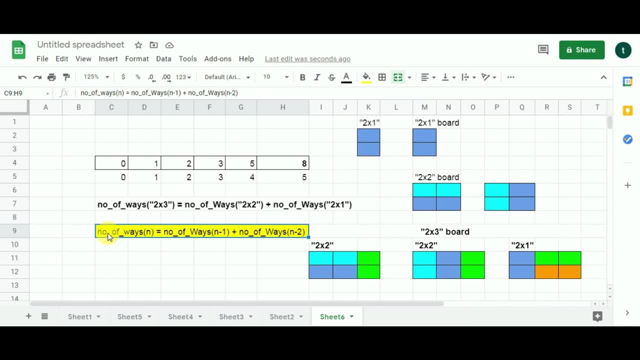 what you think of this video in the comment section. If you have any doubts regarding the explanation, do let me know in the comment section. I look so much forward to help you with programming and algorithms, And only for this video. goodbye, and take very good care of yourself, Thank you. 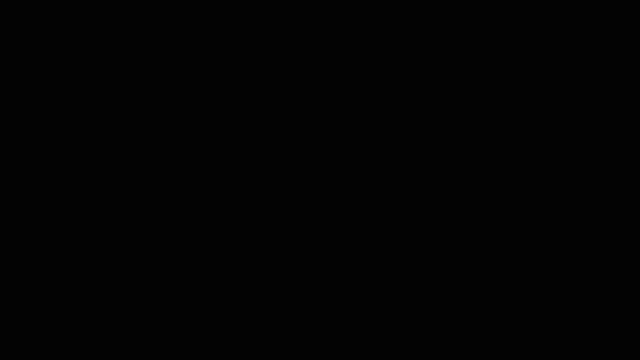 The first time you're exposed to permutations and combinations, it takes a little bit to get your brain around it. So I think it never hurts to do as many examples, but each incremental example. I'm gonna go, I'm gonna review what we've done before. 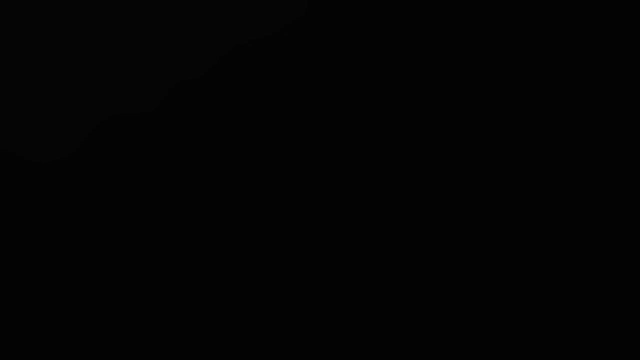 but hopefully go a little bit further. So let's just take another example, and this is in the same vein. In the next in videos after this, I'll start using other examples other than just people sitting in chairs, but let's stick with it for now.